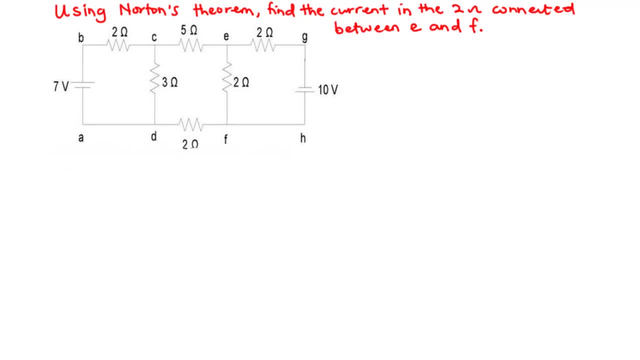 So it is sometimes difficult to find the value of current flowing through a given resistor using Norton's theorem, especially if the circuit contains more than one source. Now, if this is a challenge to you, the best thing to do is to combine Norton's theorem with. 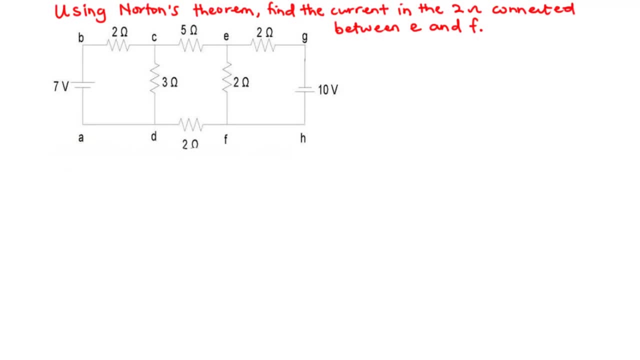 superposition theorem to find the value of current flowing through the given resistor. Now, the reason why you want to combine superposition theorem with Norton's theorem is that superposition theorem allows you to consider one of the sources at a time. Now, when you do that, you 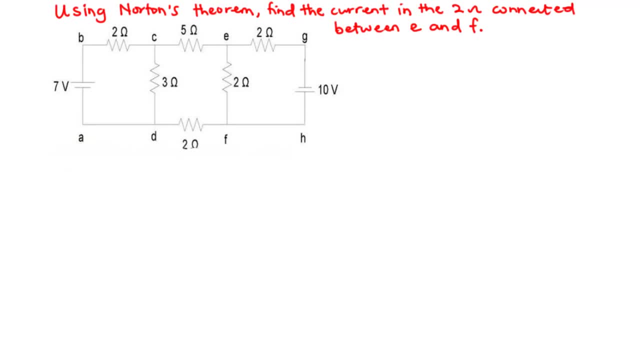 reduce the complexity of the circuit and you are able to deal with the circuit. So in today's video we are going to combine Norton's theorem and superposition theorem to find the value of current flowing through the 2 ohms resistor connected between E and F. 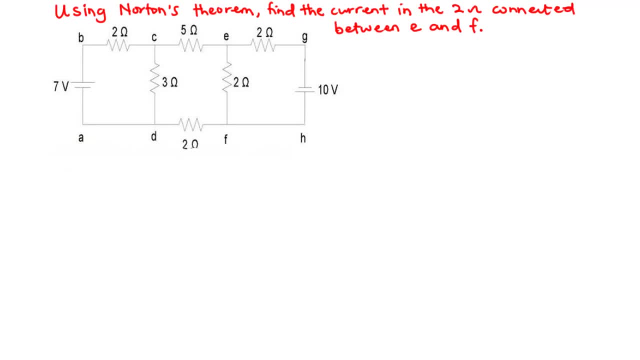 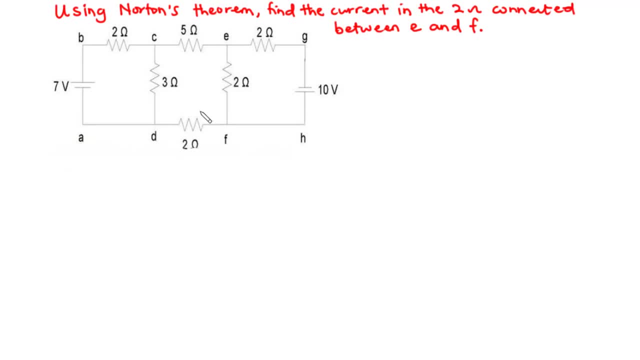 resolve this problem Now. the first thing we need to do is to resolve this problem Now. the first thing we need to do is to resolve this problem Now. when we remove the resistor, we want to find the current flowing through, that is, the two ohms resistor connected between E and 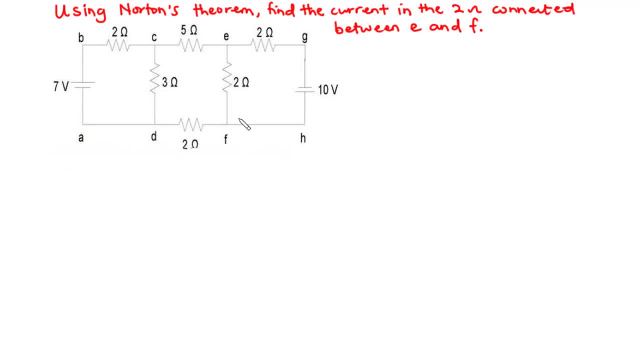 F Now, since we want to combine Norton's theorem and superposition theorem. it means Sine, we want to combine Nottings теorium and superposition theorem. it means that we need to consider one of the sources acting alone while we 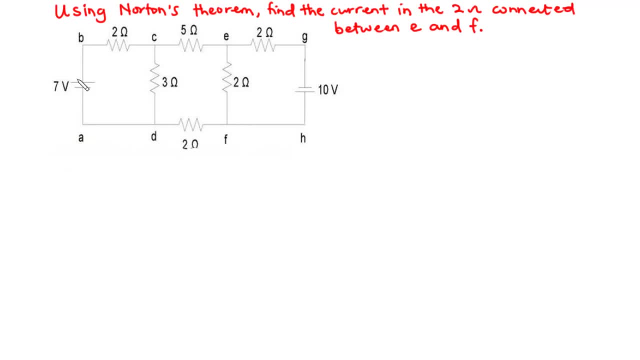 deactivate the other. So at this point we are going to consider the seven volts to be acting alone, while deactivate the ten volt source. So let 7V act alone. So let's redraw the circuit deactivating the 10V source. 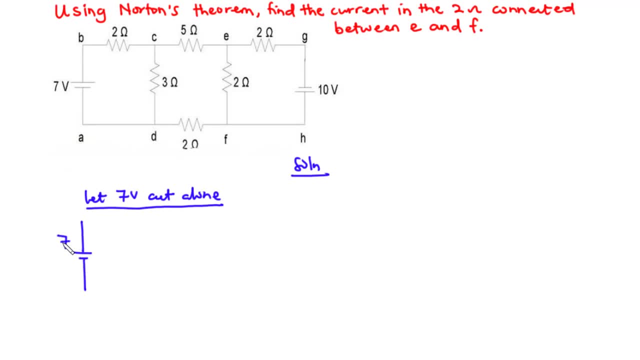 So we have this to be the 7V source. This is the 2 ohm resistor. We also have the 3 ohm resistor. We have this to be 5 ohms And then this is the short circuit current And we call that IN'. 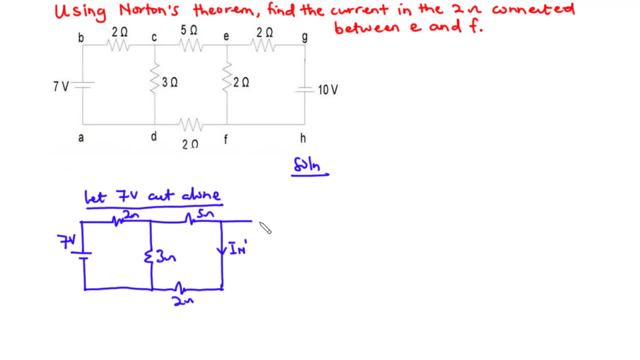 And then this is 2 ohms. We have this to be 2 ohms, And then we are going to replace this, which is the voltage source, the 10V- with a short circuit. Now, the reason why we have IN' is that we need to find the value of short circuit current. 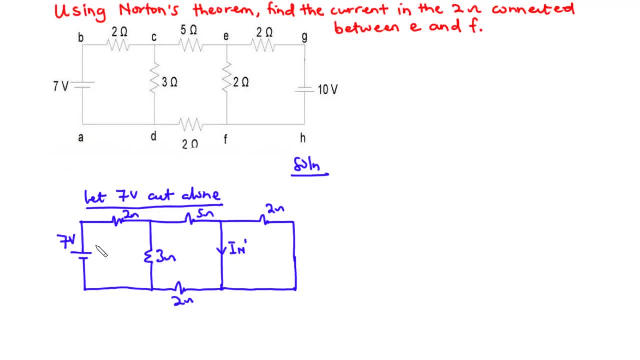 that is flowing through this branch When the 7V is acting alone. Afterwards we are going to find IN'', which is also the short circuit, current flowing through this same branch when the 10V is acting alone. So now let's find the value of current produced by the 7V. 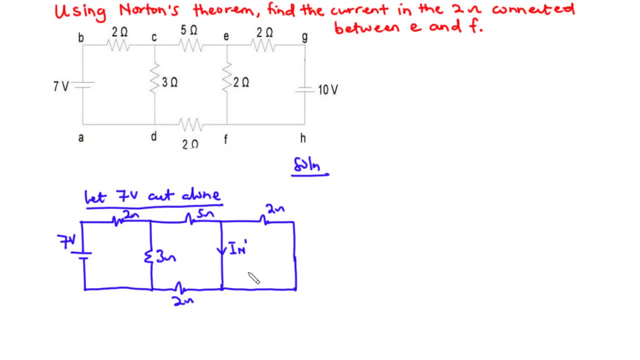 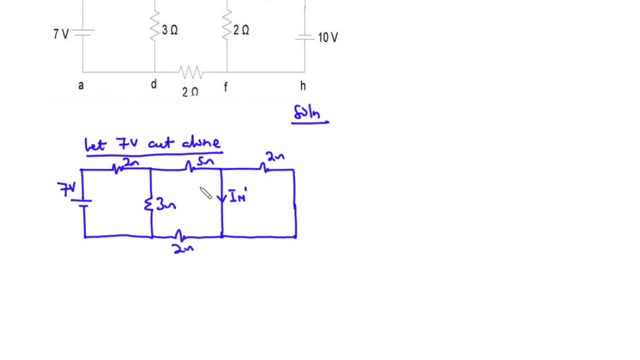 so that we can find the value of current flowing through this branch, which is IN'. So to do so, first of all let's find the total resistance for this circuit. Now you realize that when you go through this circuit we don't pass through any other circuit elements except one resistor. 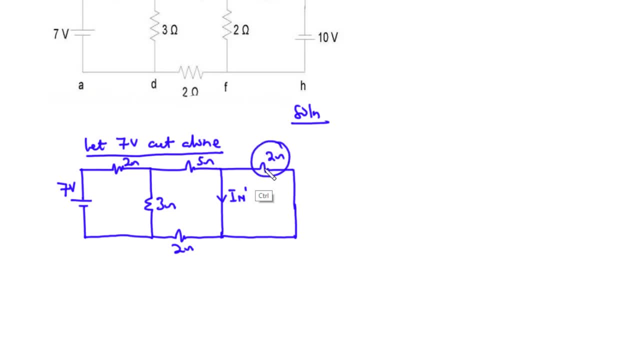 which means that this resistor has been short circuited. Therefore, in finding the total resistance, we have RT' equals. These two resistors are connected in series because the same current will flow through them and their combination is in parallel with this 3 ohms resistor. 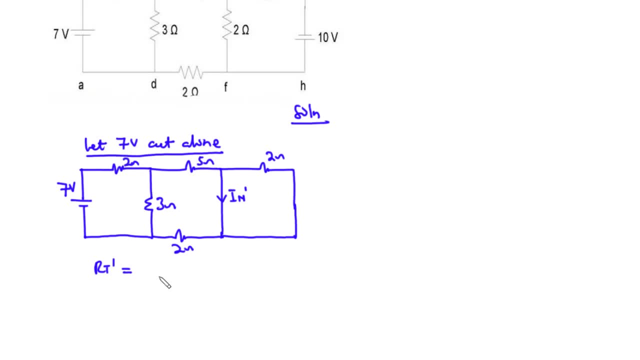 and all of that in series with the 2 ohms resistor. So we have RT' to be equal to 2 plus 5, all parallel 3 plus 2. 2 plus 5 is 7, so we have 7 parallel 3. 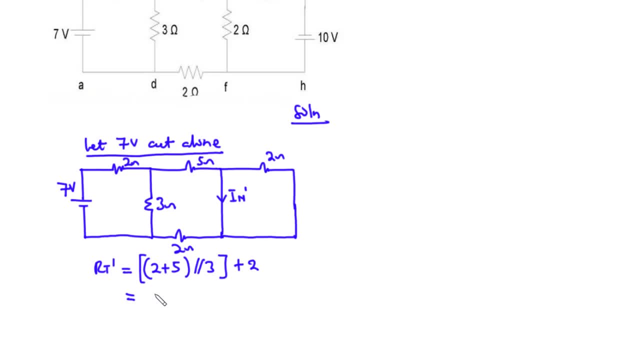 all plus 2 and then 7. parallel 3 is 2.1, so that becomes 2.1 plus 2 and that is equal to 4.1 ohms. Therefore, the value of RT' is equal to 4.1 ohms. 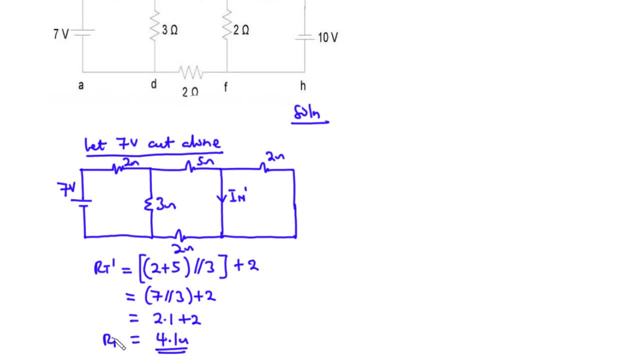 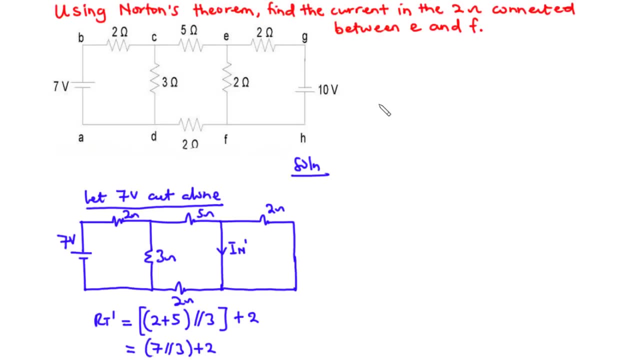 Therefore, the value of RT' is equal to 4.1 ohms. Now, since we have the value of RT', then we can find the value of current produced by the 7V source. So let's call that I' So that is the current. 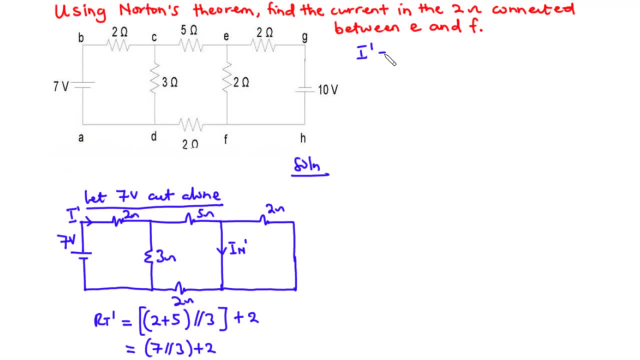 that is produced by the 7V. So I' is equal to 7 divided by 4.1, and that is equal to 70 over 41 amperes, and that is equal to 70 over 41 amperes. So this is the value of. 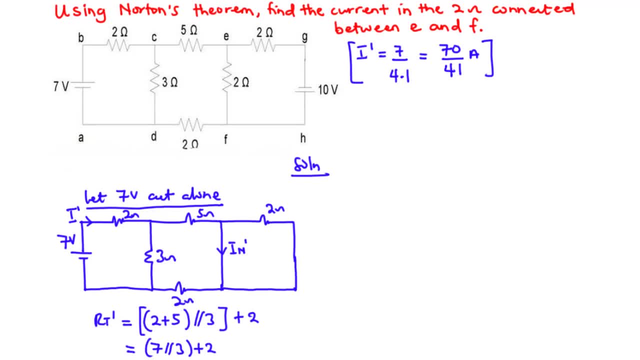 I'. Now let's move on to find the value of IN'. So IN' is equal to. Now these two resistors are in series, So their total is 7 ohms, and then we are going to distribute the current I' between this 3 ohm resistor. 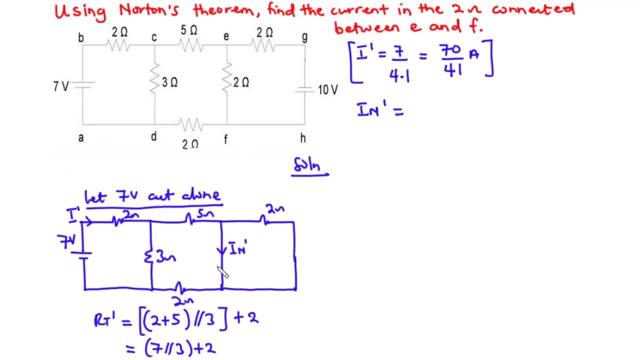 and the 7 ohm combination resistor. So the value of current that flows through these two resistors is the same current IN'. So that is equal to using the current division rule. we have the value of this resistor, which is 3 divided by the sum of the two resistors. 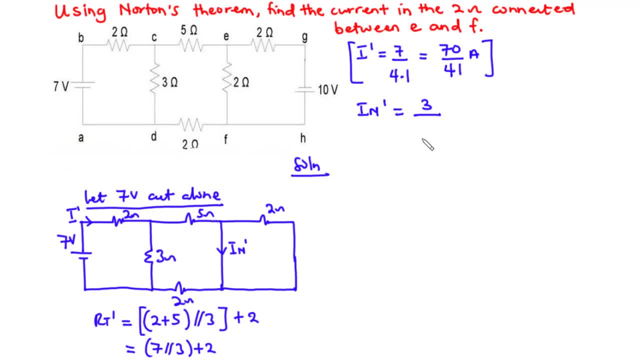 that is 3 plus the combination of these two, which is 7, So that becomes 3 plus 7 times the total value of current, approaching the junction, which is I' So times 70 over 41, and that becomes 21 over 41 amperes. 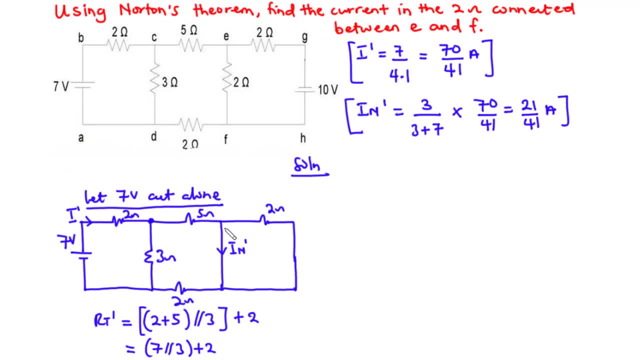 So this is the value of the short circuit current that flows through this branch when the 7 volt source is acting alone. Now notice the direction of IN' It is pointing downwards. At this point, let's deactivate the 7 volts and then consider the 10 volts. 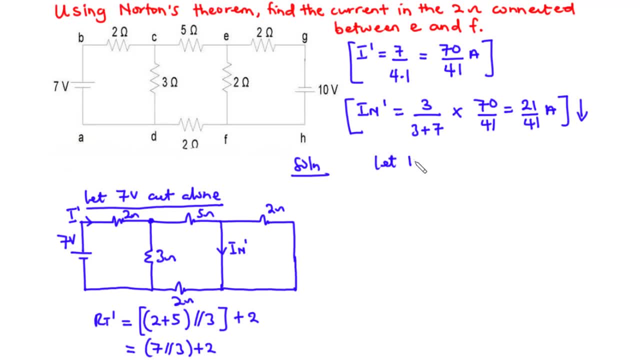 acting alone. So let 10 volts act alone. So we are drawing the circuit with the 7 volts source deactivated. We are going to represent that with the short circuit. We have the 2 ohms resistor. We have this to be the 3 ohms resistor. 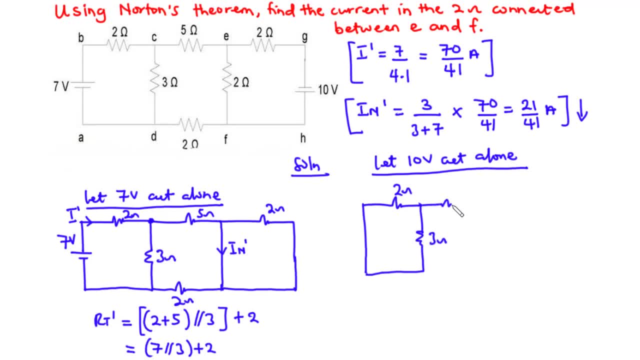 We have the 5 ohms resistor, We have the short circuit current through this branch And then this is the 2 ohms resistor. connected here We also have another 2 ohms resistor And then this is the 10 volts source. Notice the direction of current. 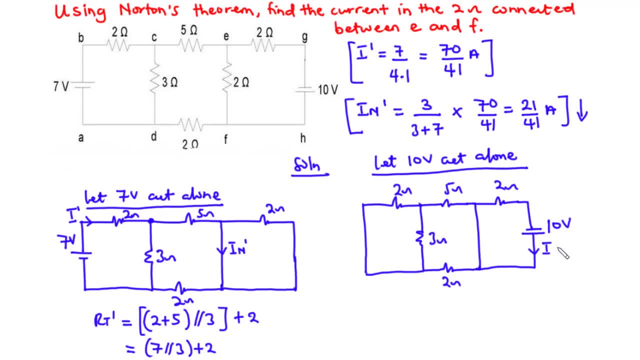 produced by the 10 volts source. Now let's call that current I'. So the current is going to move in this direction. That is the clockwise direction. Now, since we have a short circuit here, All the current produced by the 10 volts will flow through this path. 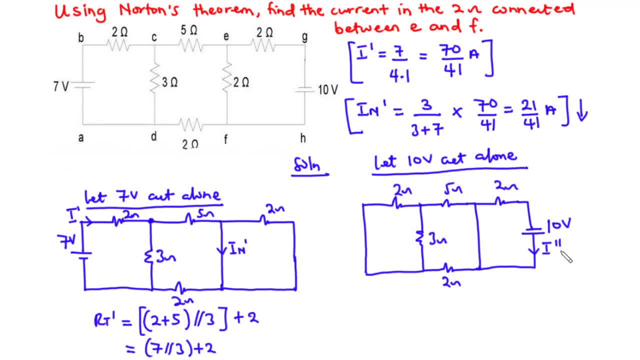 neglecting all the resistors connected here. Therefore, the current I' is the same value of current that flows through this branch and, for that matter, is equal to I N'. Therefore, I' is equal to I N' and that is equal to 10 divided by 2. 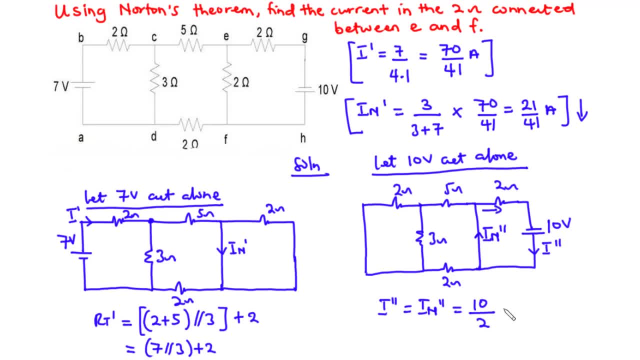 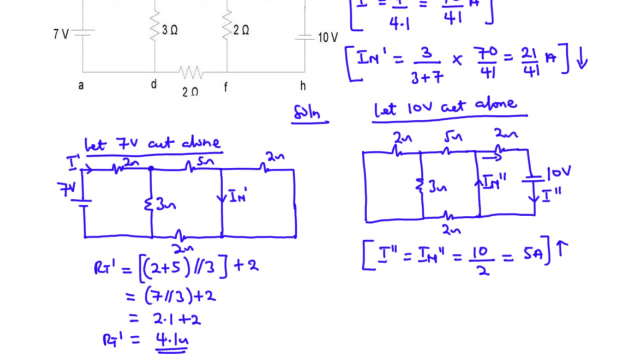 because that same current will flow through this 2 ohms resistor, and that is equal to 5 amperes. Now notice the direction of this current: It is pointing upwards. Now let's find the algebraic sum of the short circuit current I, N', and then 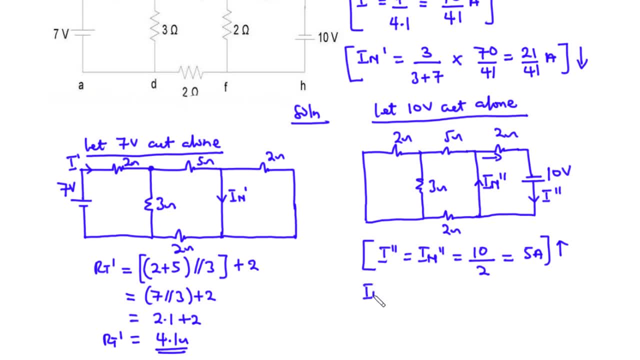 I N'. So we have I N, which is the total short circuit current flowing through this branch, and that is equal to I N' plus I N'. Now, since these 2 short circuit currents are moving opposite to each other, let's consider I N', which is flowing. 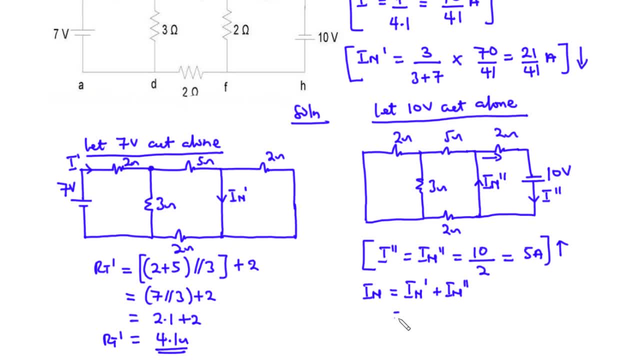 downwards to have a negative magnitude. So that would be negative 21 over 41. and let's consider the one that is I N' which is flowing upwards to have a positive magnitude. that is 5. Now when you add these 2 values, you have 184 divided by 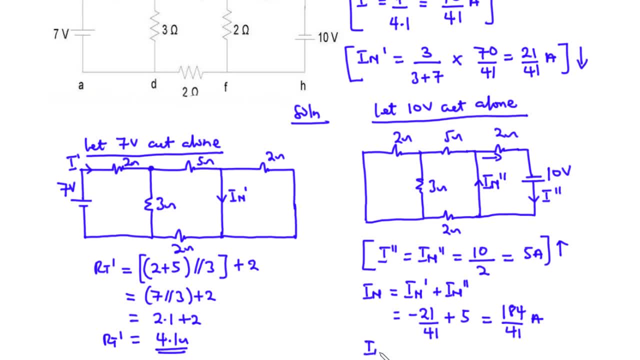 41 amperes. Therefore, we have I? N equals 4.4878 amperes. So this is the total value of short circuit current flowing through this branch. Now, since we have the value of I N, let's move on to find the value of R N, which is: 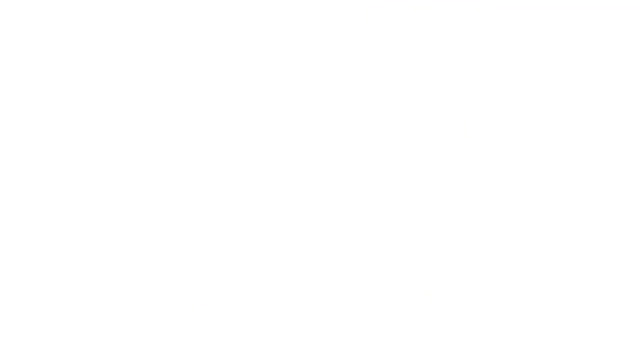 the N' resistance. So to find the N' resistance, R, N, we need to redraw the circuit, deactivating all the sources. and because we have voltage sources, we are going to replace them with short circuit. So the 7V is replaced with a short circuit. 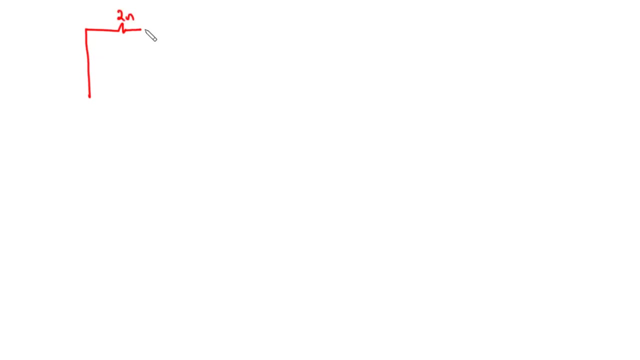 We have this to be the 2 ohms resistor. We also have the 3 ohms resistor, We have this to be the 5 ohms resistor, And then this is the terminal A B. We also have this to be 2 ohms, And then we also have 2 ohms. 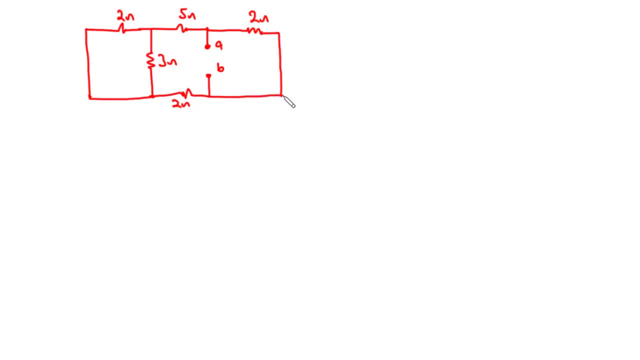 And then we have a short circuit And then we complete the circuit. So to find the value of R N. These 2 resistors are connected in parallel And their combination is in series with the 5 ohms resistor and also the 2 ohms resistor. 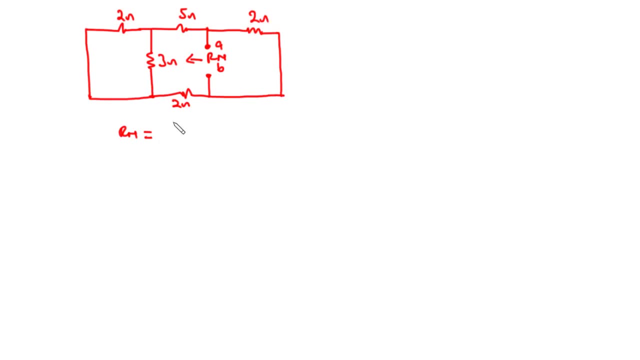 And all of that in parallel with this 2 ohms resistor. Therefore we have 2 parallel 3, all plus 5 plus 2, all parallel 2. Now 2 parallel 3 is 1.2, 1.2 plus 7 is 8.2. 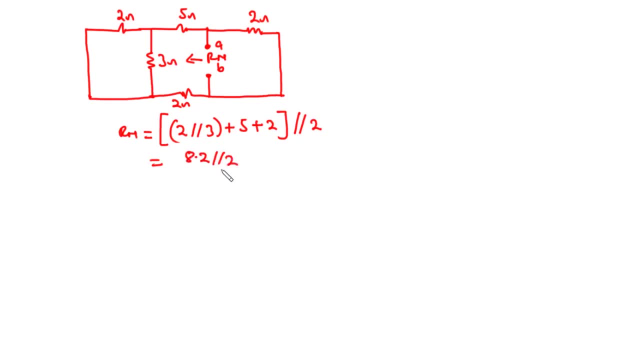 So we have 8.2 parallel 2, And then 8.2 parallel 2 gives 1.6078 ohms. 1.6078 ohms, So this is the value of R N Now, since we have the value of I, N and then R N. 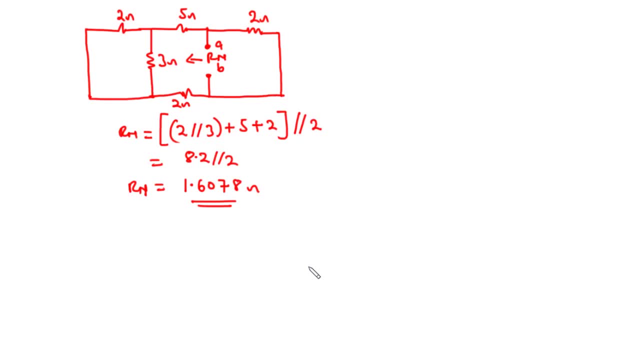 We can find the value of current flowing through the 2 ohms resistor connected between the 2 terminals. So let's draw the Norton's equivalent circuit. So we have this to be the short circuit current. I N Notice that we had the greater magnitude of current. 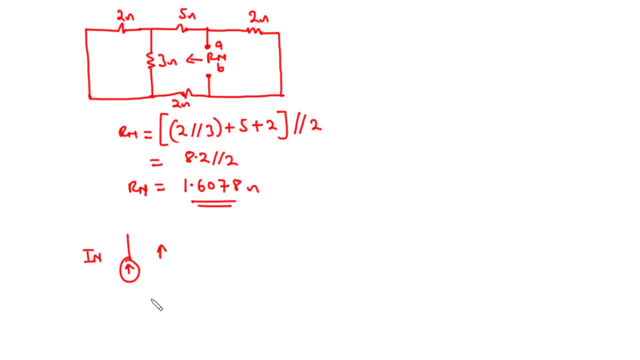 flowing this way, which means that the total short circuit current I N will also flow in this direction. that is R N. So we have this connected in parallel with the Norton's resistance. that is R N. And then we also have the load resistor, that is the 2 ohm resistor. 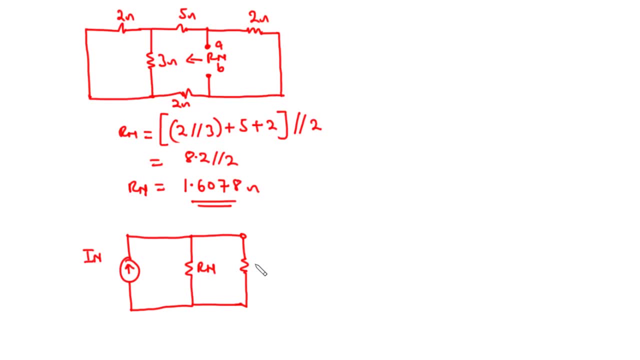 connected in parallel with R N. So that is R L equals 2 ohms. So we had I N to be 4.4878 amperes And then we have R N to be 1.6078. Now to find the value of current flowing through. 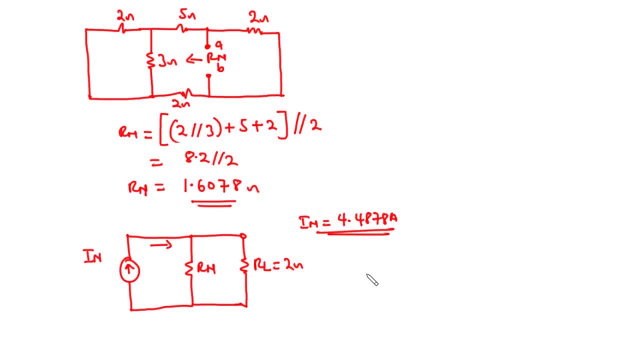 the 2 ohms resistor. We are going to use the current division rule, So the value of current flowing through the 2 ohms resistor is equal to the value of this resistor, which is 1.6078 divided by the sum of the 2 resistors.